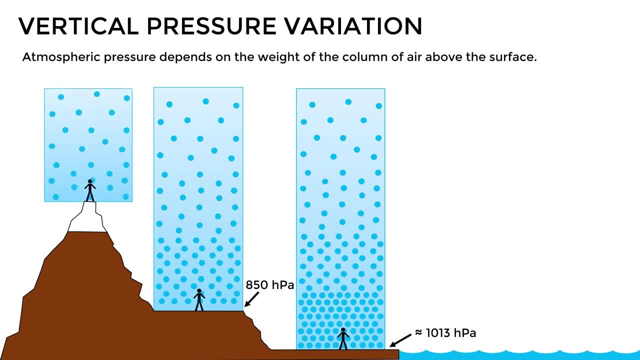 for example, to the top of this mountain, there will be even less air above us and therefore the pressure will be considerably reduced, obtaining values of around 500 hectopascals. So, in summary, we can say that the higher the altitude, the lower the pressure. 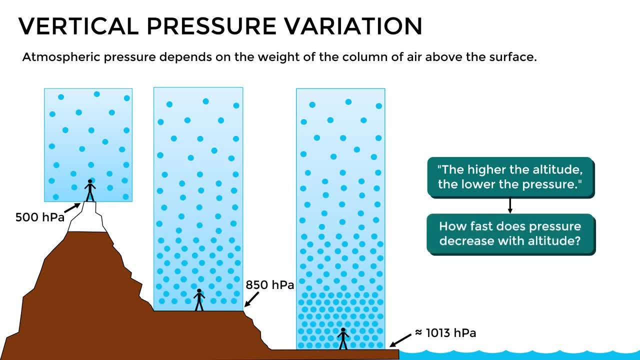 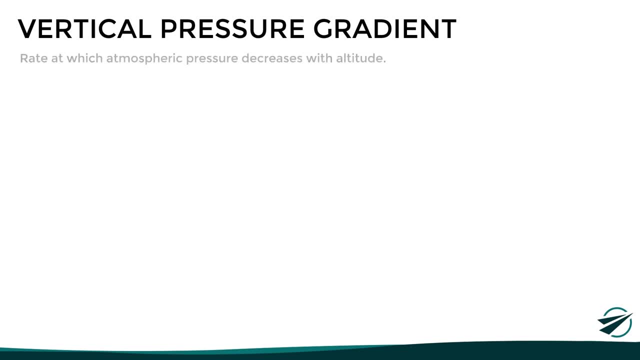 But the question now is: how fast does atmospheric pressure decrease with altitude? Well, to answer that, we have to look at the vertical pressure gradient, which is a parameter that basically measures the rate at which atmospheric pressure decreases with altitude. However, if we want to measure the rate at which atmospheric pressure decreases with altitude, we 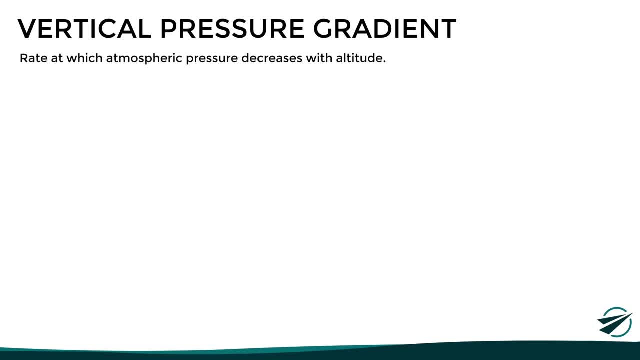 have to look at the vertical pressure gradient. As we said in the video about the composition of the atmosphere, there is no defined boundary between the atmosphere and space, so for this example, we will assume that this boundary is 100 kilometers. So, with this in mind, 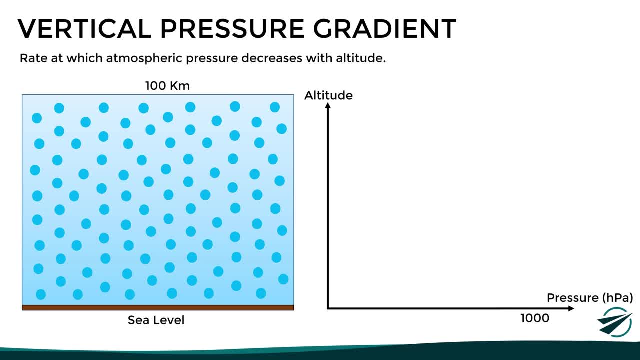 and taking into account that the pressure at sea level is around 1000 hectopascals, one may think that if we climb up to the middle of the atmosphere, which in this case is 50 kilometers, then the pressure would be half of what we had at sea level around. 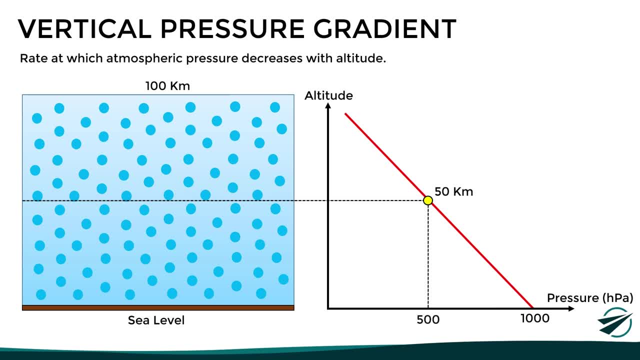 500 hectopascals. This sounds logical, since at this point we would only be supporting half the weight of the atmosphere, But we have to say that this is just not true. This is because air is a compressible fluid, which means that most of it is concentrated in the lower levels of the 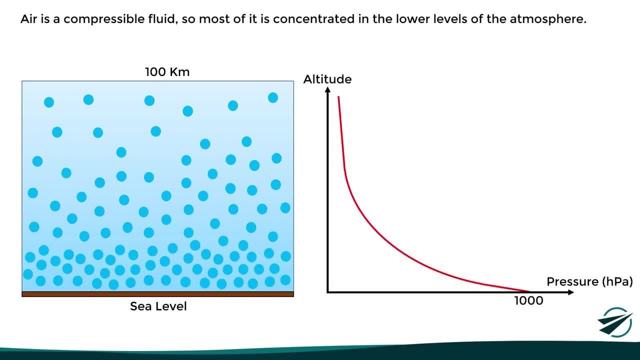 atmosphere. This way, we would rather obtain a graph like this, where the pressure reduces a lot faster at low altitudes than at higher levels. This means, in other words, that pressure does not decrease at a constant rate, and therefore we can say that the vertical pressure gradient changes. 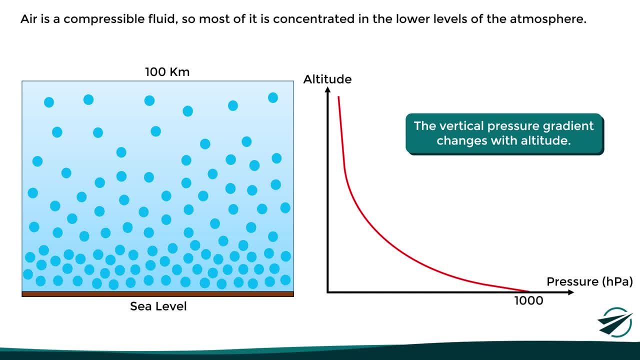 with altitude. For example, if we were to climb to an altitude of only 5.5 kilometers or 18,000 feet, the atmospheric pressure would drop by about a half, reaching values of around 500 hectopascals. And if we continue climbing up to 10 kilometers or 33,000 feet, 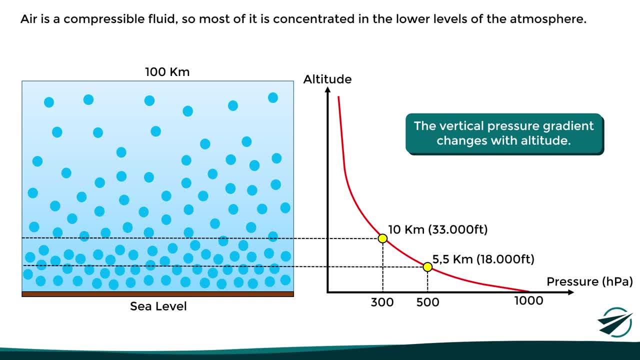 then the pressure would be reduced to about one third of that of sea level. Now, while it is true that the rate at which the pressure changes with altitude is variable, the truth is that at the lowest levels, typically below 10,000 feet, this rate is relatively 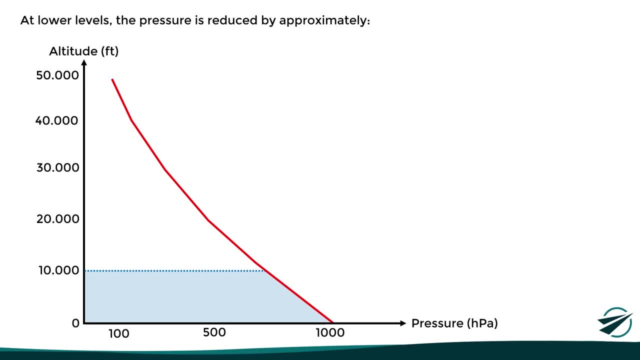 constant. In fact, we can say that the pressure here is reduced by 1 inch of mercury per thousand feet, or 1 hectopascal per 30 feet. Now this vertical pressure gradient not only varies with altitude, but also with air temperature. To understand, 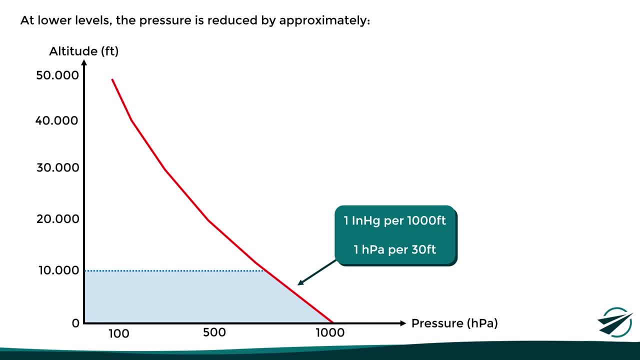 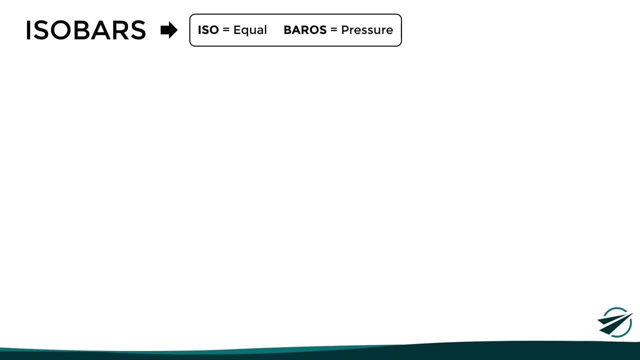 this better. let's first look at a concept that is pretty useful to analyze the behavior of pressure, which are the isobars. This is a Greek term meaning equal pressure, And therefore these are lines joining points of equal pressure. So, with this in mind, let's look at how we can. 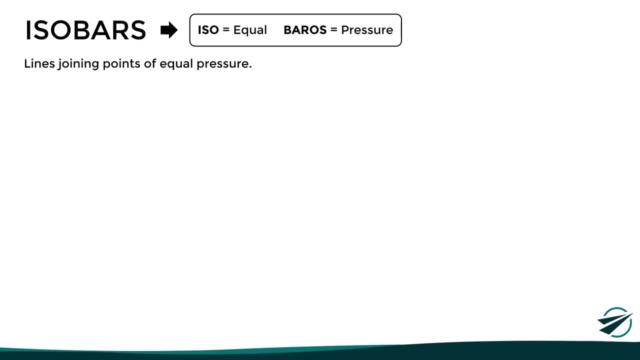 analyze the vertical pressure gradient using these isobars. Here we have the mean sea level, where the pressure is around 1013 hectopascals. This means that the 1013 isobar will be located at an altitude of 5,000 feet. Now if, for example, at an altitude of 5,000 feet we get a pressure of 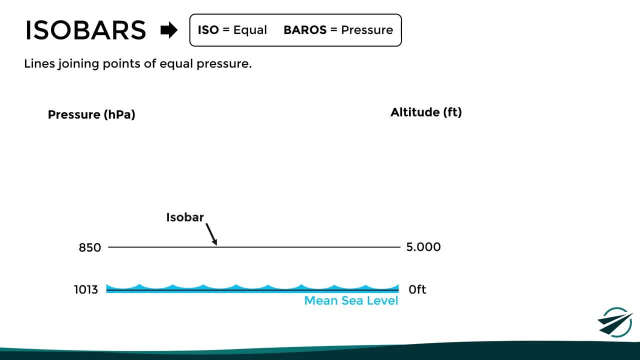 850 hectopascals, then we can draw the 850 isobar at that level And if we continue with this order of ideas, at 10,000 feet and 15,000 feet we would find the 700 and 570 isobars respectively. 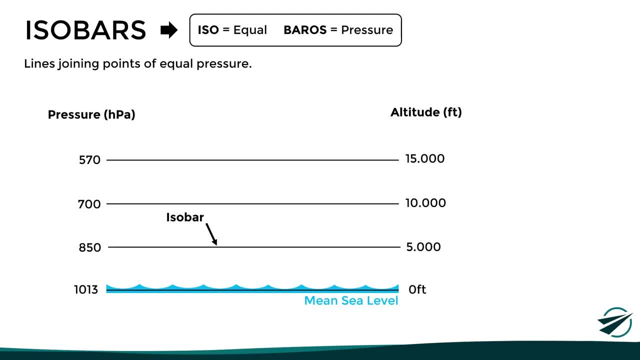 Now, it is important to bear in mind that these pressure values are found only under standard conditions, Since, in practice, temperature variations can affect the position of these isobars. But you might be wondering: what does the position of these isobars have to do with the 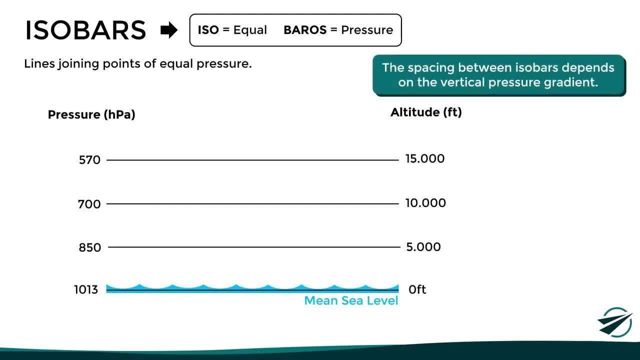 pressure gradient. Well, the spacing between isobars depends directly on the vertical pressure gradient. For example, if the isobars are closer together, then it means that the pressure changes rapidly with altitude, or in other words, we have a high vertical pressure gradient. 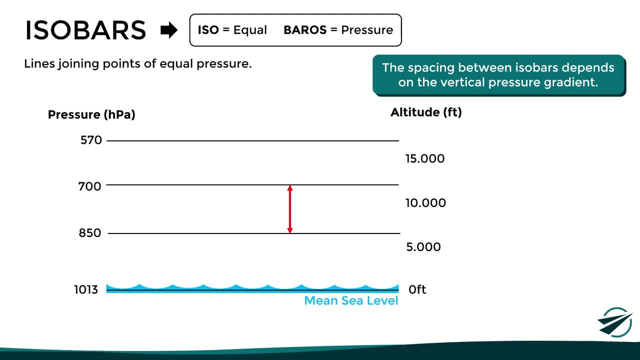 On the other hand hand, if the isobars are widely spaced from each other, this means that the pressure changes slowly with altitude and therefore we have a low vertical pressure gradient. It is important to note that the spacing of the isobars has nothing to do with the pressure. 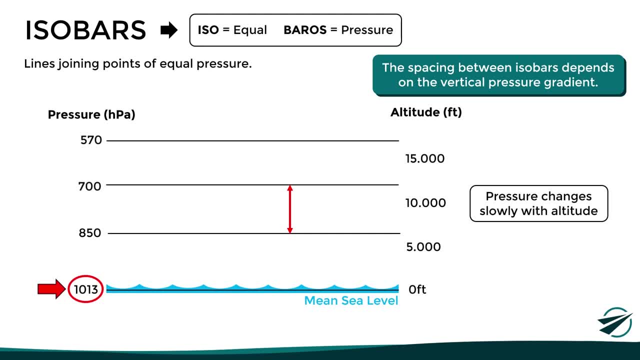 at sea level. In fact, in both cases the pressure at sea level remained constant at 1013 hectopascals. The only thing that changed was the rate at which the pressure decreased with altitude. So you might ask: what does the spacing of the isobars depend on? Well, in most cases, 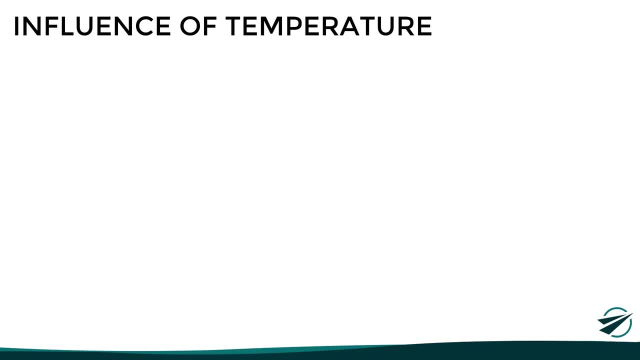 the answer is air temperature. The thing is that air temperature affects air density and therefore it also affects the pressure distribution with altitude. In general terms, the higher the temperature, the lower the vertical pressure gradient, and vice versa. For example, under standard temperature conditions at sea level pressure is reduced by 1 hectopascal. 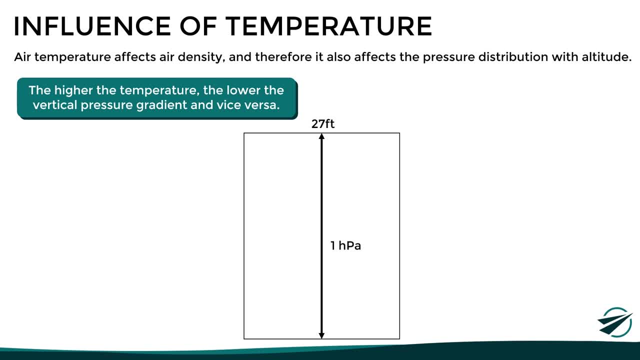 for every 27 feet. However, if the temperature is higher than standard, this will cause the air to expand and therefore have a lower density. This in turn causes the pressure to reduce more slowly with altitude. In this particular example, the pressure is now reduced by 1 hectopascal. 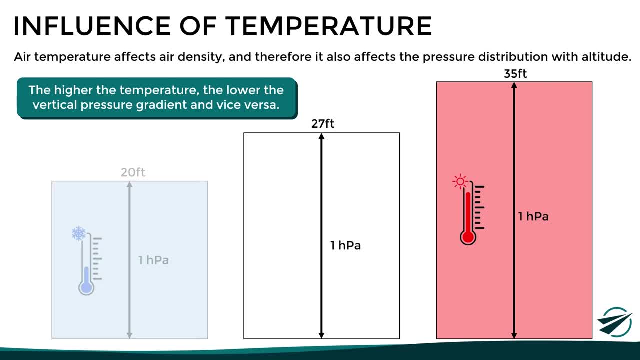 for every 35 feet. On the other hand, if the temperature is lower than standard, then the air will shrink and therefore will have a higher density. This in turn causes the pressure to change more rapidly with altitude. In this example, the pressure is now reduced by 1 hectopascal for every 20 feet. 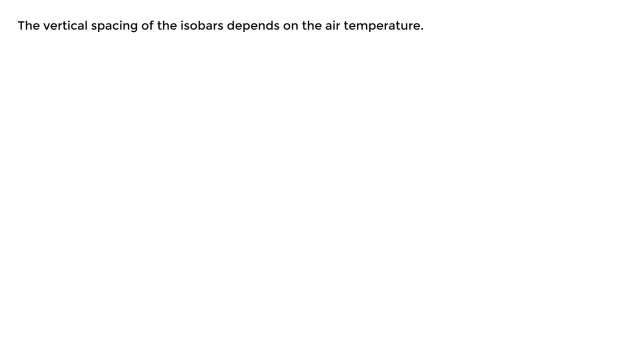 All this implies that the vertical spacing of the isobars depends on the air temperature. For this example, we will have a constant pressure at sea level of 1013 hectopascals. So here we can see how the isobars would behave in a column of air under standard temperature. 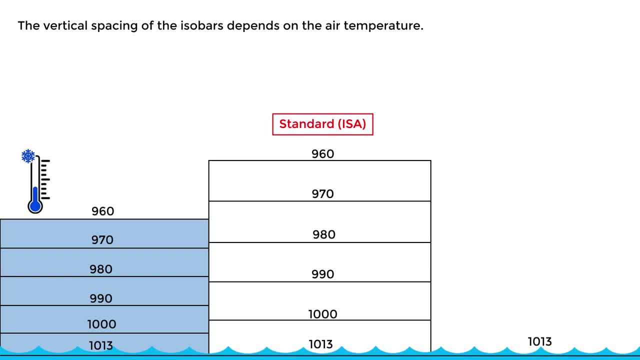 conditions. On the left, we can see how the same isobars would behave with a lower than standard temperature, where the pressure reduces more rapidly with altitude. And finally, on the right, we can see how those isobars would be arranged with a higher than. 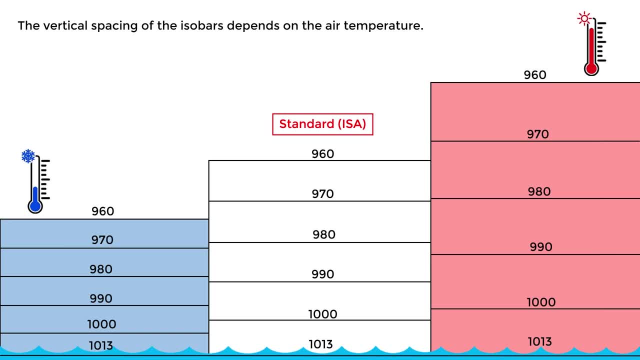 standard temperature, where the pressure changes slowly with altitude. Now, something to note here is that the pressure at the bottom and at the top of all three columns is the same. However, the heights of the columns are different because of this difference in the pressure distribution. This means that the pressure at the bottom and 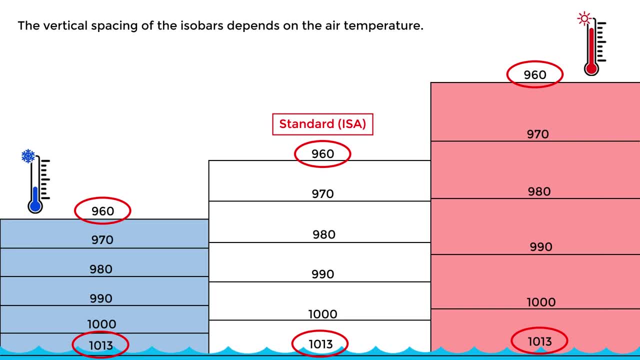 the height of the column is different. Actually, this is the reason why barometric altimeters suffer from temperature error, which we have already discussed in the videos about flight instruments. Now, so far, we have focused on how pressure changes with altitude. It is now time to see. 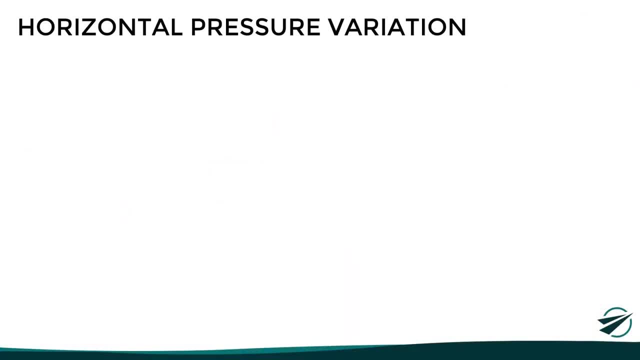 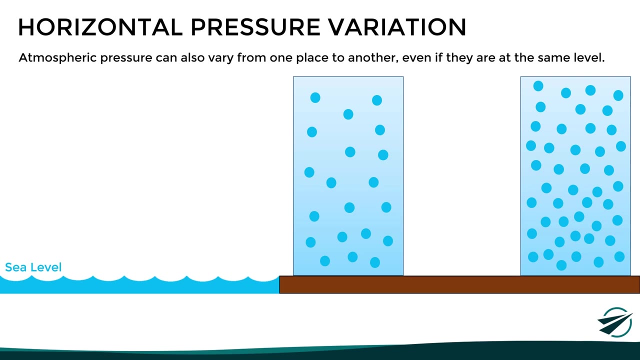 how pressure changes horizontally with distance. As we said before, atmospheric pressure can also vary from one place to another, even if they are at the same level or altitude. In this case, principle applies: In the areas where there is less air above the surface, there will be a lower. 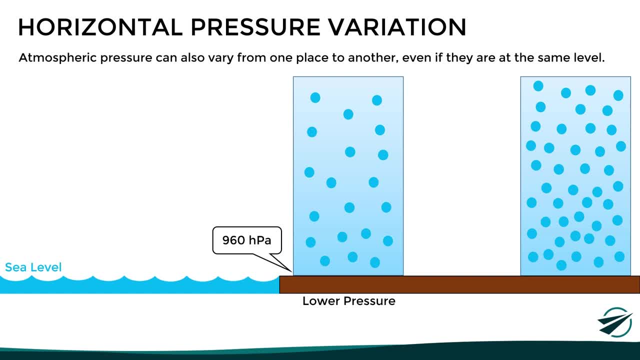 pressure, While in the areas where there are more air molecules above the surface, the pressure will be higher. But you might be wondering: if these two columns have the same height, why don't they have the same amount of air? Well, the answer is, once again, air density. In this case, the column 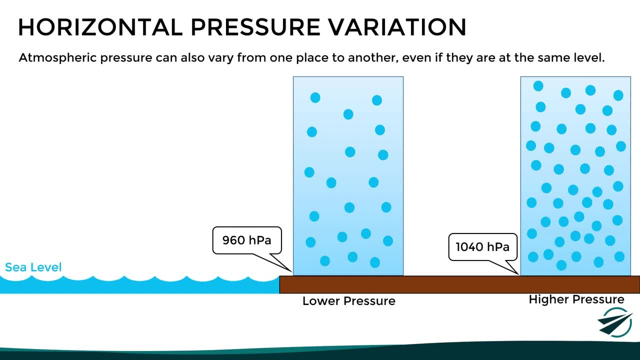 of air on the right has a higher density than the one on the left, which results in different atmospheric pressure values at the surface. These density differences are mainly due to temperature variations and the movement of large air masses caused by global atmospheric circulation, But we will not go into detail on this subject in this video. For instance, let's look at what 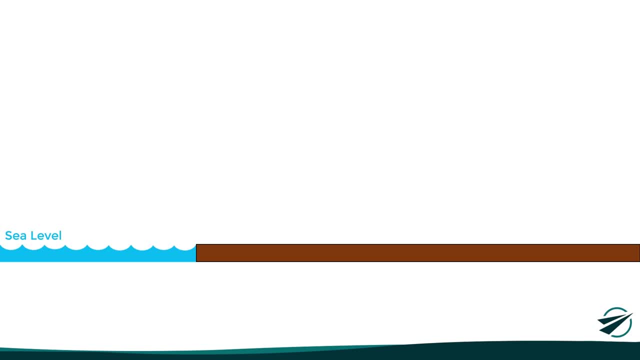 happens when there are horizontal pressure differences. Let's say there are three places that are at the same level and in each of them we have a barometer to measure atmospheric pressure. So at point A let's say that we have a pressure of 960.. At point B we have a pressure of 1005.. And at point 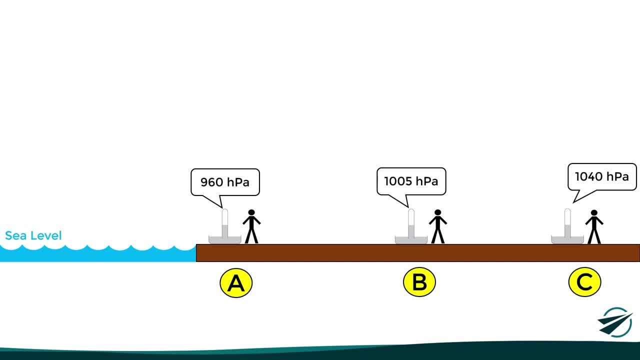 C, we have 1040.. With this, we can easily say that point A is an area of relatively low pressure, which is identified with the letter L, while the point C is an area of high pressure, identified with the letter H. So in this situation, if we move from point C towards point A, even though we 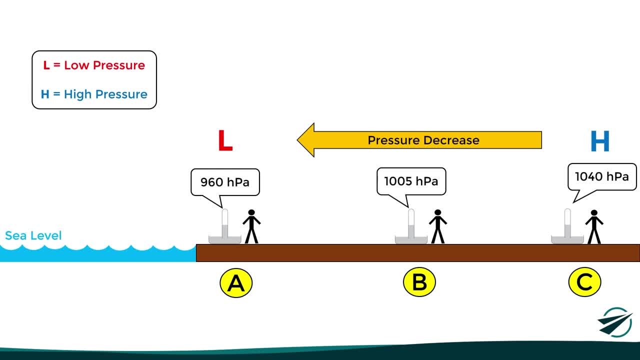 remain at the same level or other pressure. we have a pressure of 960.. At point B, we have a pressure of 960.. And if we use the particle structure in this case for altitude, we will experience a decrease in pressure, While if we move in the opposite way, we will see an increase in pressure. Now the question. 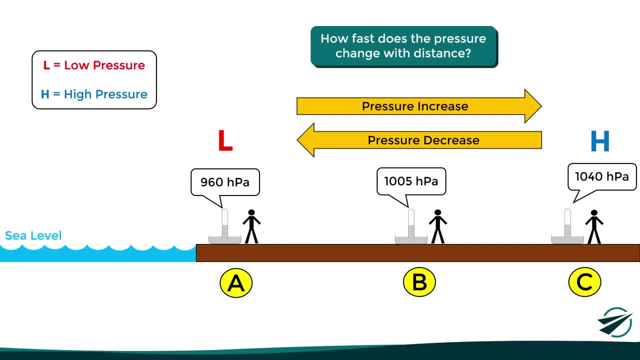 is: how fast does the pressure change with distance? Well, in the same way as we analyze the pressure change with altitude by means of the vertical pressure gradient, we can do exactly the same in this case, looking at the horizontal pressure gradient, which is basically the rate. 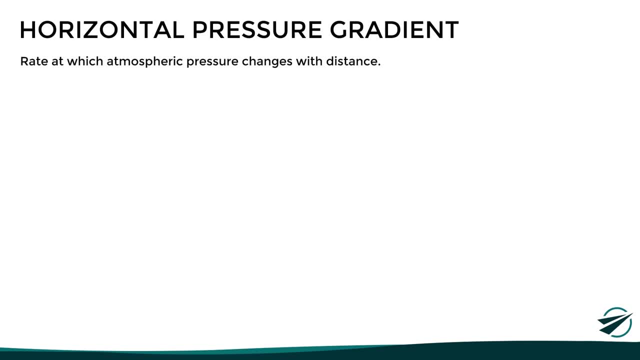 which atmospheric pressure changes with distance. For example, let's say that in this case, point A has a pressure of 960 and point B a pressure of 1040.. Now it is evident that the pressure difference between these two places is 80 hectopascals. 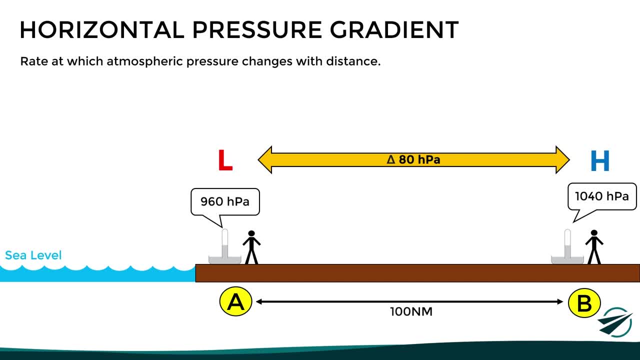 and let's say that the distance between them is 100 nautical miles. Well, with this information, we can easily determine the horizontal pressure gradient by dividing 80 by 100, thus obtaining a gradient of 0.8 hectopascals per nautical mile. 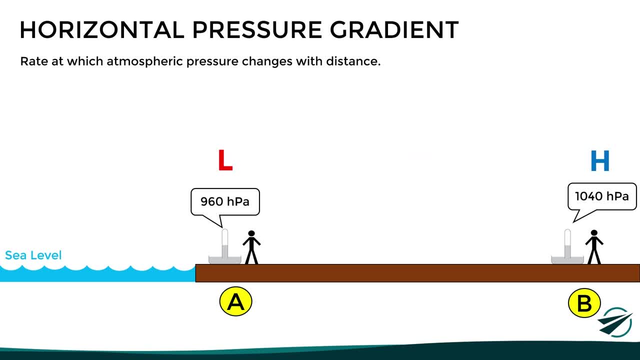 Now, in this situation, if the distance between these points were shorter, let's say 50 nautical miles, then the horizontal pressure gradient would be twice as high, resulting in 1.6 hectopascals per nautical mile, which in the end, means that the pressure changes more rapidly with. 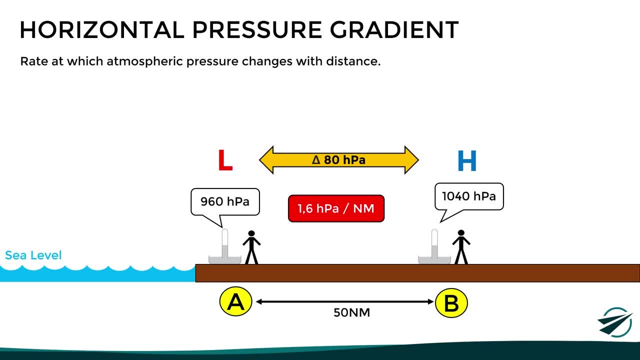 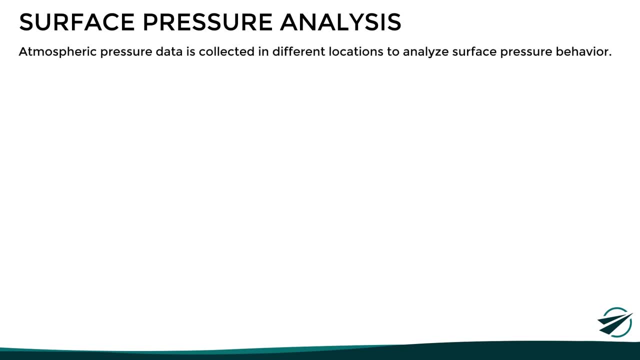 distance. Now, the analysis of how pressure changes with distance at the surface is referred to as surface pressure analysis. In order to do it, atmospheric pressure data is collected in different locations to analyze the surface pressure behavior. For example, let's say we have this big island and we have different weather stations distributed. 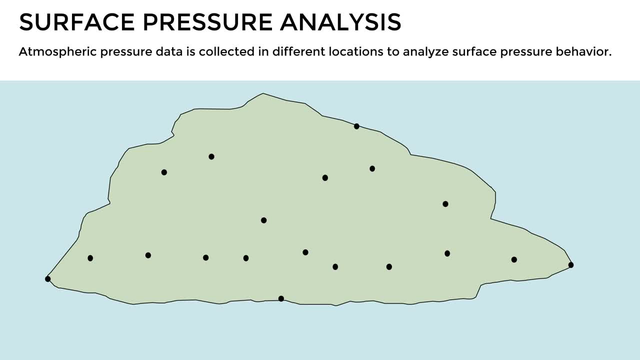 at different locations but at the same level. Now let's say that at 10 am all these stations report their local atmospheric pressure simultaneously. Initially we can identify two important places: The area with the lowest pressure and the area with the highest pressure. 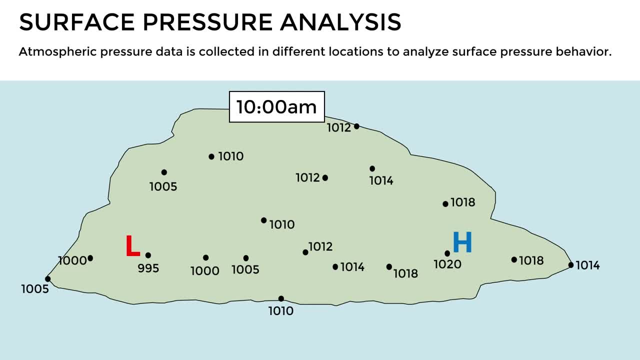 Now, what if, to better analyze the pressure behavior, we join with a line the stations that are reporting exactly the same pressure? These lines, by definition, are isobars, but instead of being used to measure the vertical pressure gradient, we are now using them as reference for the horizontal pressure gradient. 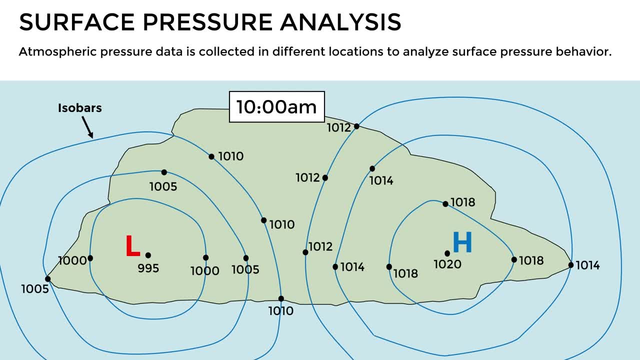 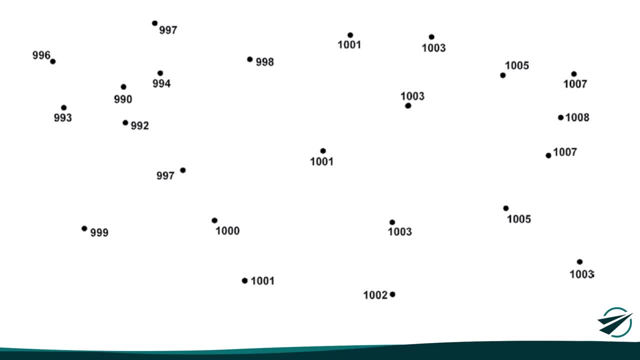 As we can see by drawing these isobars, we now have a much clearer idea of how the pressure behaves at the surface. In this other example, we can see exactly the same thing. Initially it looks like a series of dots and numbers without much meaning. 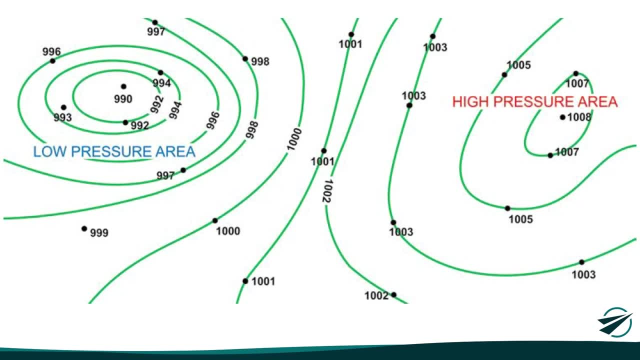 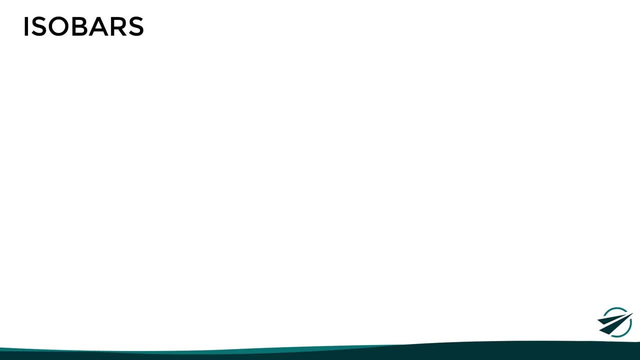 However, once we draw the isobars, we see that there are concrete pressure patterns on the surface. Now, just as we used isobars to analyze pressure vertically, we can also use them for the horizontal pressure gradient. Let's say, for example, that we have point A with a pressure of 960 and point B with a. 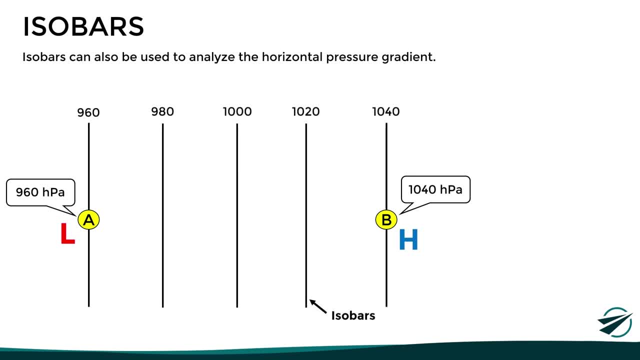 pressure of 1040.. In between we can see the isobars that determine how fast the pressure changes with distance. This way, if the isobars are widely spaced apart, then it means that there is a low horizontal pressure gradient and therefore the pressure changes slowly with distance. 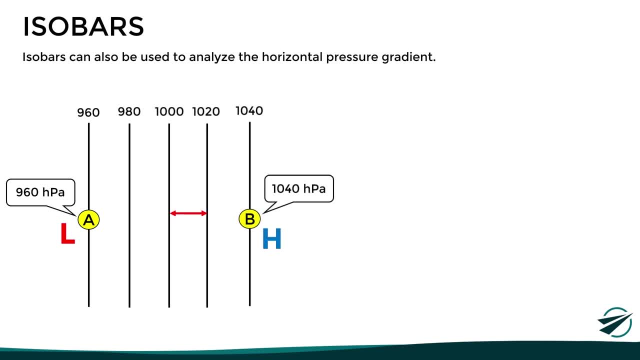 While, on the other hand, if the isobars are closer together, then it represents a higher horizontal pressure gradient, resulting in a more rapid pressure change with distance. At this point, you might think, why is it important to analyze pressure in the first? 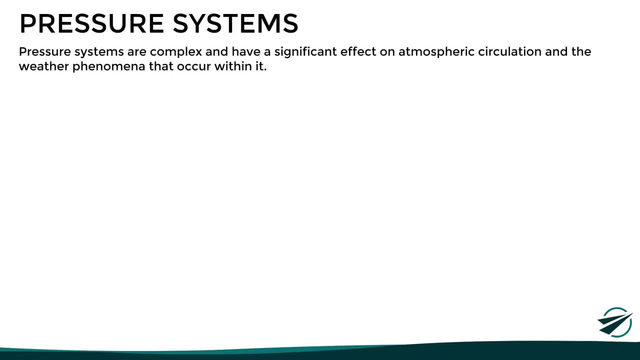 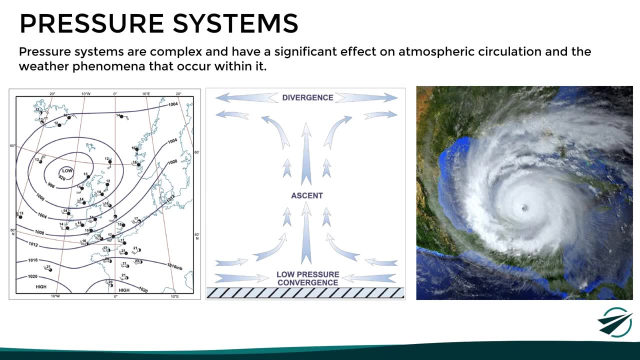 place. Well, pressure systems are complex and have a significant effect on atmospheric circulation and the weather phenomena that occur within it. Most meteorological phenomena have something to do with pressure behavior, but we'll talk about that in a future video. Before finishing, we must look at one last concept. 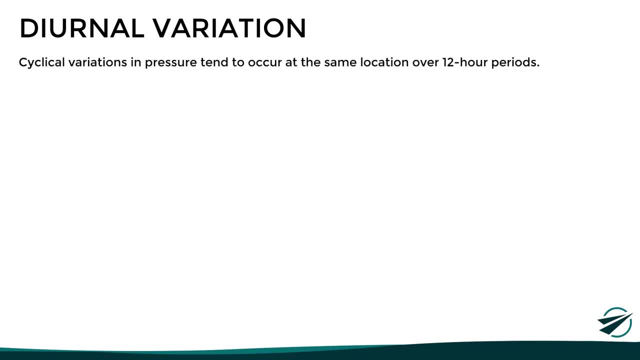 The diurnal pressure variation And is that in the same place there tends to be cyclical variation? Yes, There are cyclical variations of pressure in periods of 12 hours. These pressure changes show a relatively predictable pattern, with the highest pressure values. 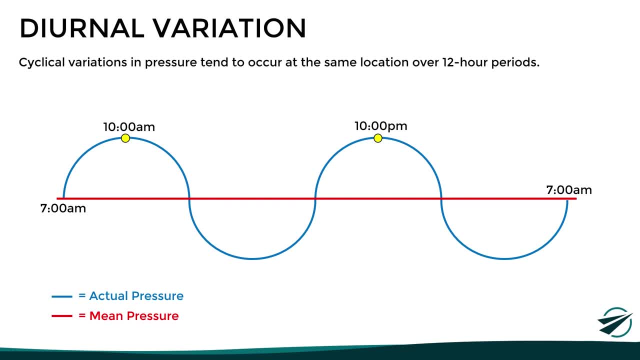 found around 10 am in the morning and at 10 pm in the evening, while the lowest pressure tends to be found around 4 am in the morning and 4 pm in the afternoon. Now, it is important to mention that these diurnal pressure variations are usually maximum. 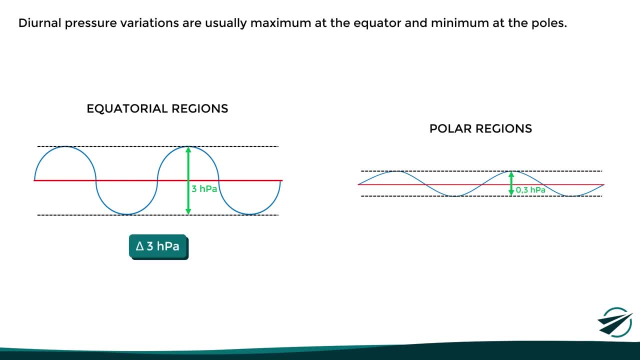 at the equator, where the difference between high and low pressure is around 3 pm per minute, And they tend to be minimum at the poles, where the typical variation is around 0.3 hPa. However, it is important to mention that the atmospheric pressure at a certain location